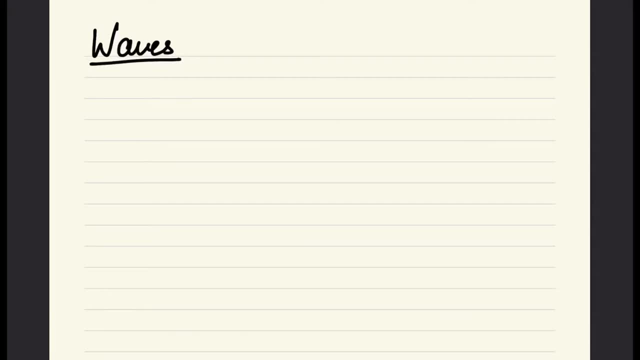 Hello everyone, I hope you'll be fine. So I'm back again with the next topic on all-level physics, and this is about the waves. So since my previous videos, the syllabus has been changed now, and now I'm gonna start off with this topic like waves, and then 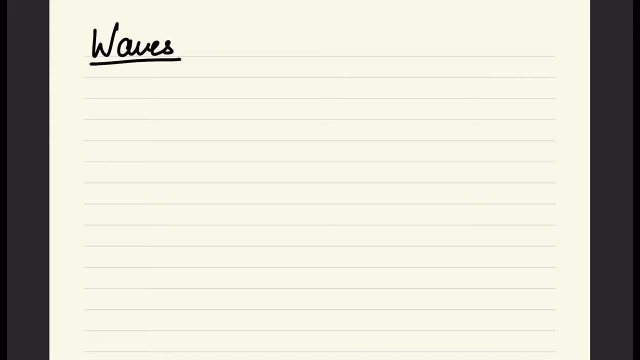 we'll have like some more topics. So from now onwards I'm gonna proceed with the new specifications as it has been given in the GCSE Cambridge curriculum. So in this topic, in this chapter of waves, we have four subtopics. Number one is about the general properties of the waves. So in 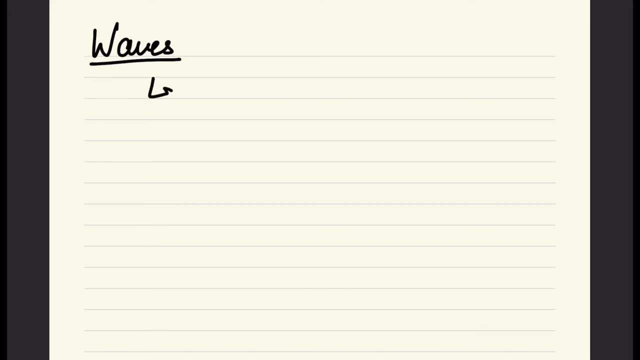 this topic, first of all we'll discuss about the general properties of waves. So in this topic we'll discuss just about the general properties of the waves, and then comes the light, and then we'll discuss about the electromagnetic spectrum, and after that, in the end, we will discuss about the sound. the sound. 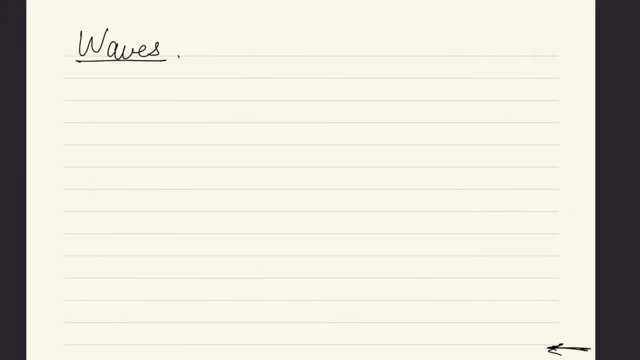 waves. So in waves, first of all, we have to discuss, like, what are the waves and why are they used? So, basically, the waves are used to transfer the energy from one point to another, without transferring the matter. Alright, so I'm just gonna write it over here: Waves are used to transfer energy from one point to the. 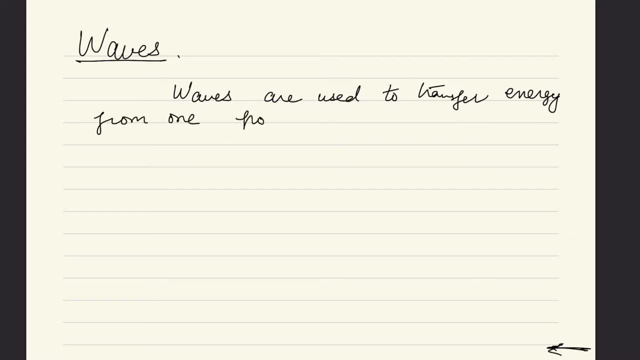 another without transferring the matter. So these are the waves. For example, let's suppose there is a string that is attached to a wall like that: This is the wall and this is the string. We move the string up and down from this. so as the spring moves up and down, it transfers the energy from this point over that point all. 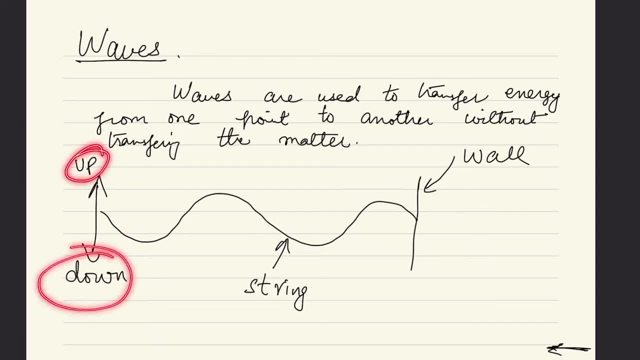 right. so basically, as we move the spring up and down, the energy is being transferred from this point to that point in the form of wave. so that's how we can explain why, how the energy is transferred from one point to another point. all right, now let's take another example. so, for example, we 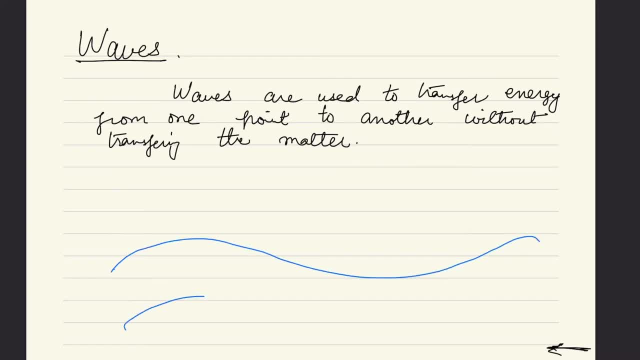 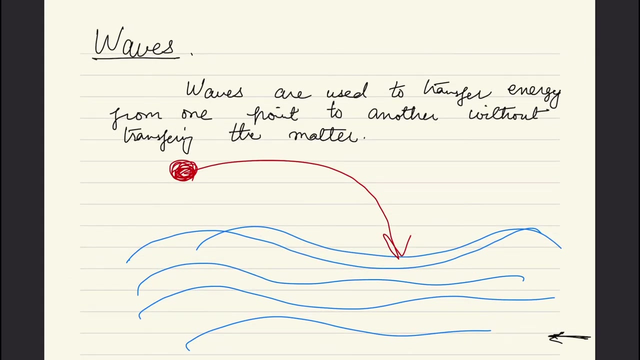 have water surface over here. this is water, right, and someone throws a stone into the water, all right. so when a stone is thrown into the water, circular waves will be formed over here, like that. so these waves, they will spread out, and that's how the energy is transferred from this point in the outward direction. so after this introduction, let's. 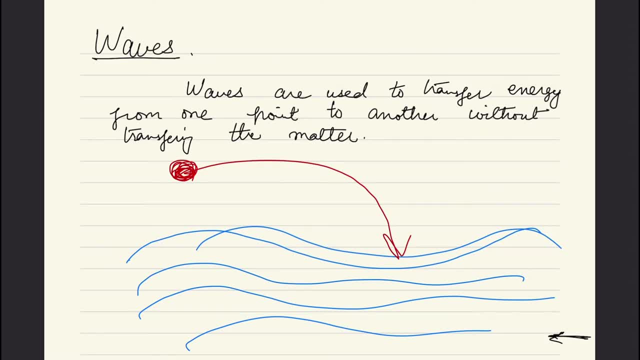 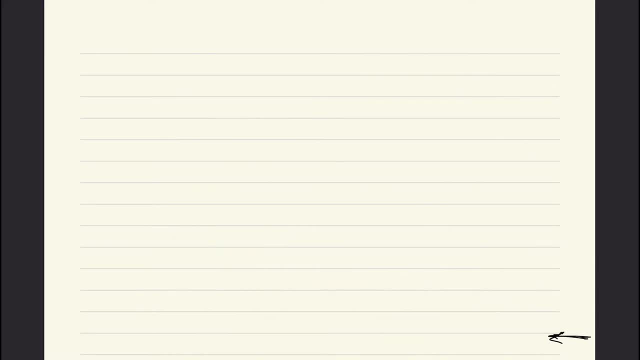 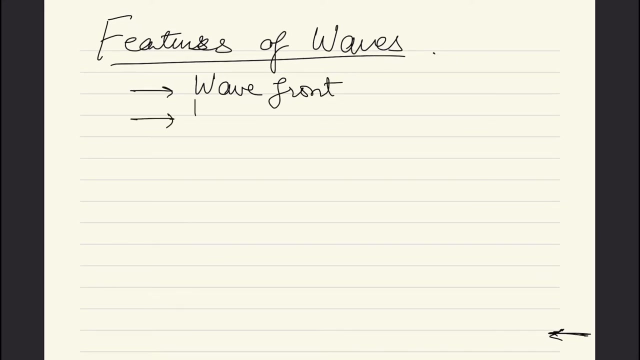 discuss some of the features of a wave. so it is it all, and we'll discuss some of the features of the waves, features of waves. so in these features, you have to discuss wavefront, you have to discuss the wavelength, then comes frequency and then we have to check the wave speed. so, in order to discuss these features one by one, let me 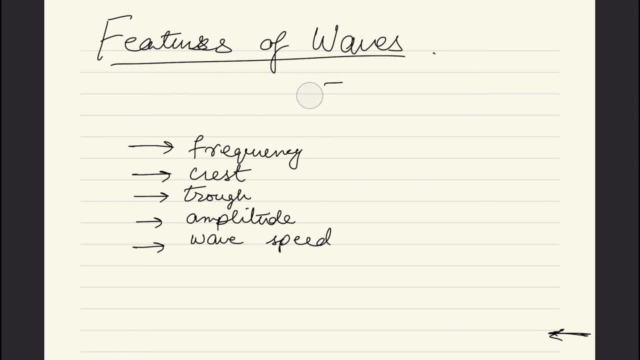 just start off with the wavefront. so for the wavefront, for example, this is a wave. if you see this wave from top, it will look like this. so this is the Top view And this is the side view Of the wave. Alright, now observe it carefully. 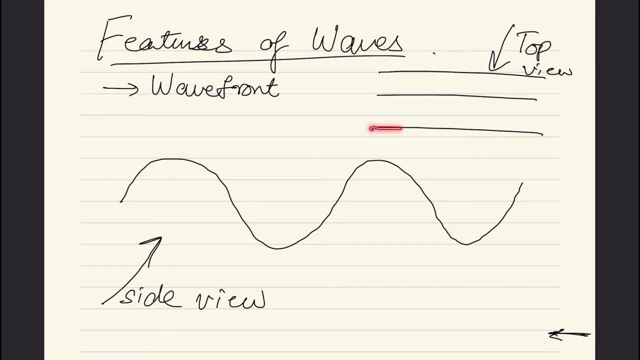 This point over here is being represented by this line, This point over here is being represented by this line, And This point over here is being represented by this line. So these are called the Wavefronts right, So in other words, The tops or the peaks of the wave. 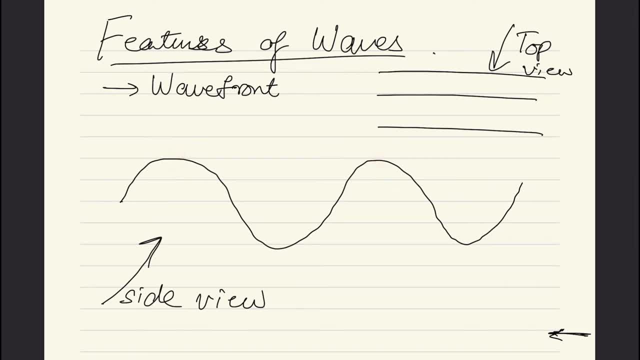 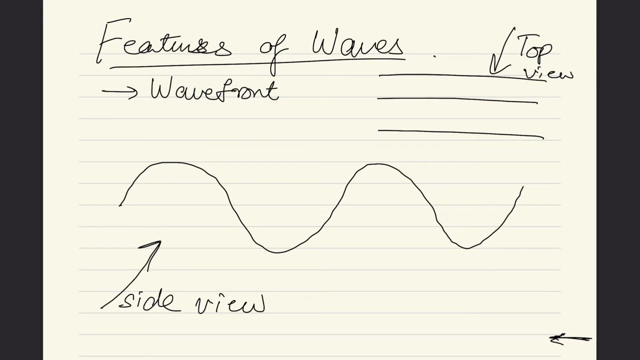 They are the wavefronts, Alright, so whenever we see the wave from the top, These lines will represent the peaks And The region exactly in between these lines will represent These lower peaks. We'll discuss the top peaks and lower peaks in the next features. Okay, so the next feature. 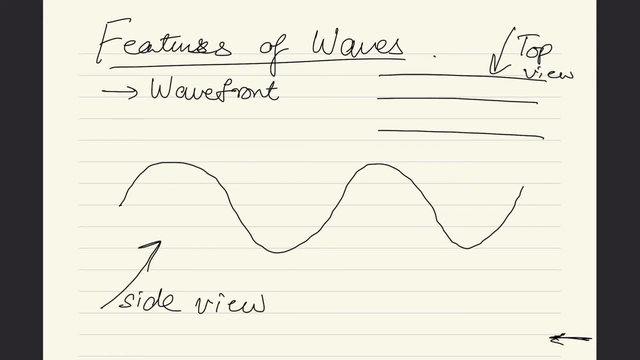 That we have to discuss is the wavelength. So, for example, I have drawn a wave over here. So the length from this point All the way to this point, Or the length from this point Or this point, Or the length from this point, of the wave To this point. 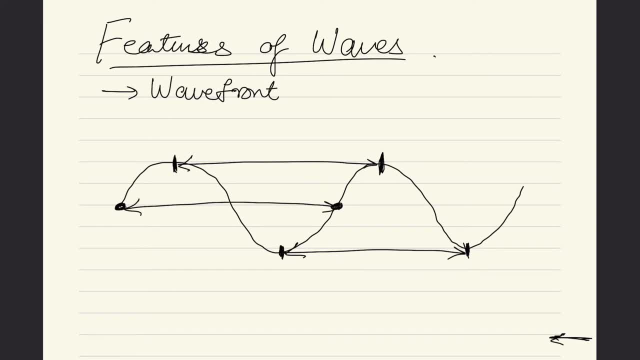 To this point, They are all the same length And they are called the wavelengths. But before that, I want to explain you About the Crest And trough This Positive peak that you are seeing. This is the crest, This is the crest And This bottom peak that you are seeing. 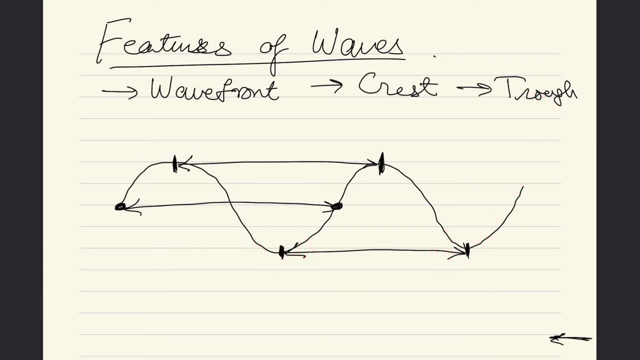 These are the Truffles. So the positive peak is the crest And the negative or the bottom peak Is the trough. So the distance between two consecutive Crests Or the distance between the two consecutive troughs Is called the wavelength, Or The distance That a wave completes in one cycle. 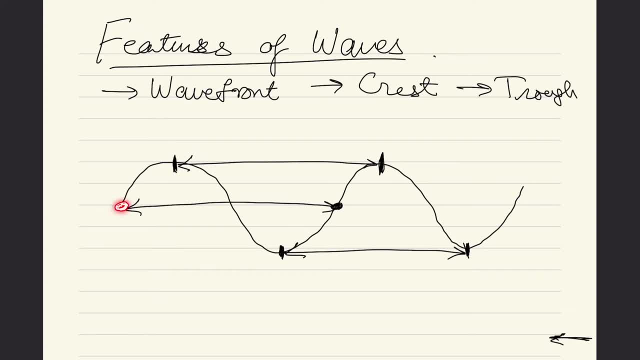 Is the wavelength. So the cycle of the wave starts from here. There is the quarter cycle, Over here, half cycle, Three, fourth of cycle And a complete cycle. So that's why the distance From the beginning to the end Of the cycle Is called the wavelength. Alright, So we are discussing about the wavelength. 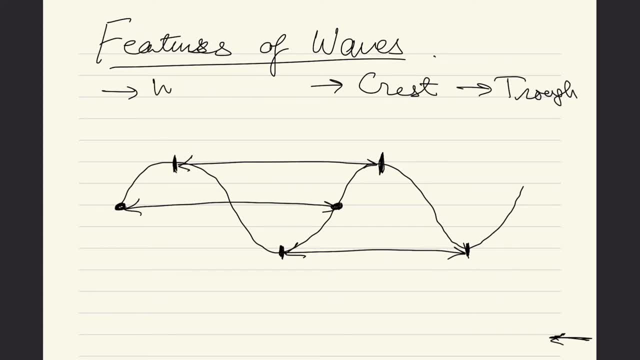 So let me just write wavelength over here. So Crest, as I told you, Is the positive peak, trough is the negative peak And wavelength is basically- Let me just write down the definition over here- The distance Between The distance Between The distance Between two consecutive Crests, Crests. 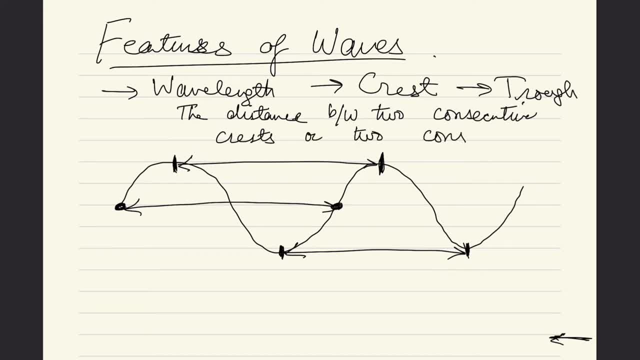 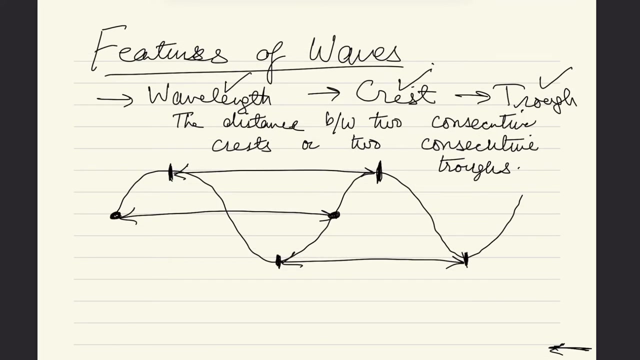 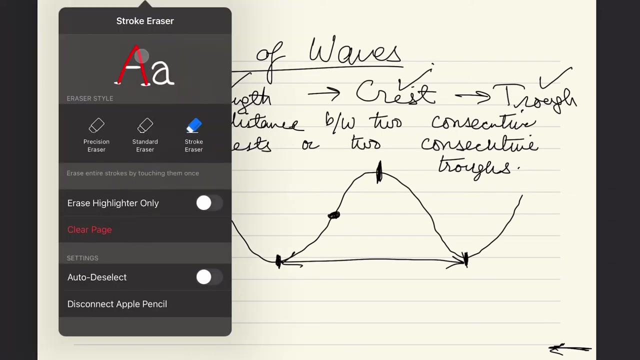 Or Two consecutive Truffles, Truffles. That distance Is called the wavelength. Alright, So we have discussed three more features of the wave: Wavelength, Crest and trough. So the next feature of the wave That we have to discuss Is the- Let me undo it. So The next feature that we have to discuss, 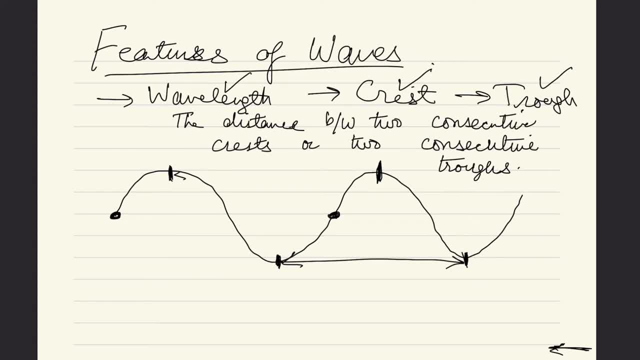 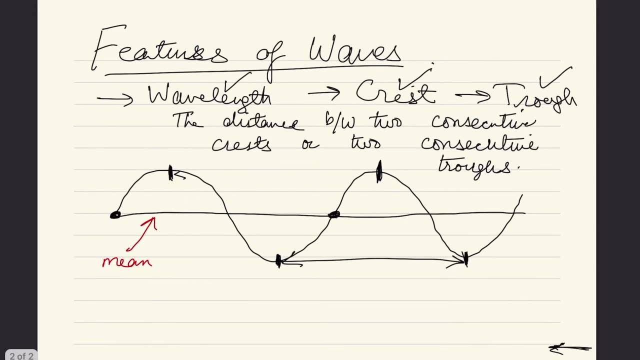 Is the amplitude. So Let's suppose this is the middle of the wave. Amplitude is basically the distance. Okay, basically, First of all we have to check, We have to discuss the position. So this position of the wave is the Mean position And this position over here, That's the 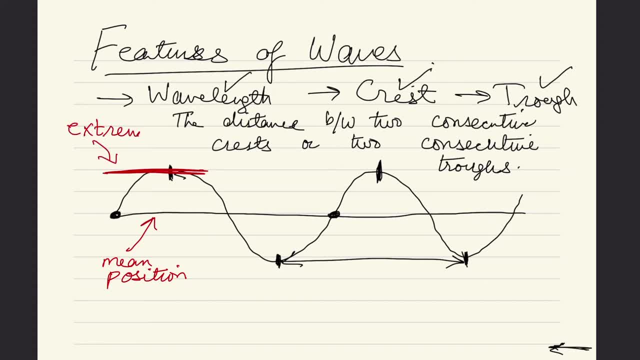 Extreme position. Similarly, This is The okay. so this is the positive Extreme and that's the negative Extreme. positive extreme, Negative extreme. Now, amplitude is basically Amplitude is the Distance between the positive Extreme and the negative extreme. So we can say That the distance From the mean position. 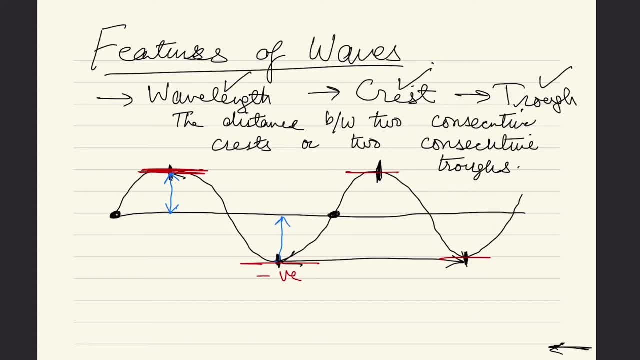 To any of the extreme Position is the Amplitude. So these blue lines Are representing the Amplitude. So that's the amplitude Of the wave. By definition, we can say that The distance Between The Mean position And Extreme position Is the amplitude Right. so this is the Definition for the amplitude. 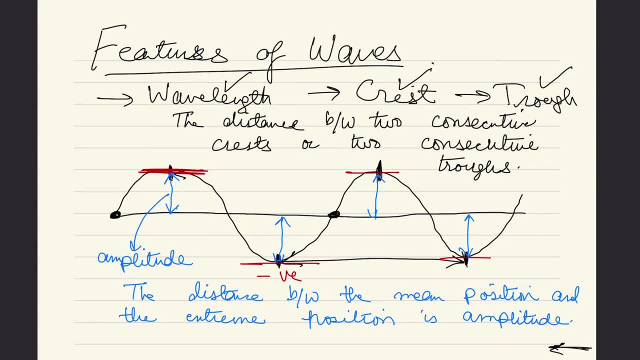 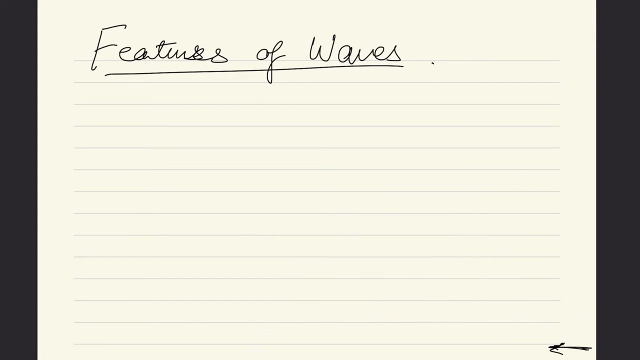 So this is another feature Of the wave. So after amplitude, we have to discuss The wave speed And the frequency. So let's move on towards the Frequency. Let me just raise it down So I'll explain you. frequency By it's definition: Frequency is Basically The number Of cycles. 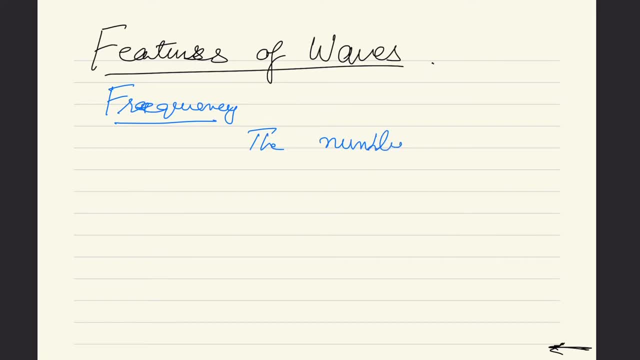 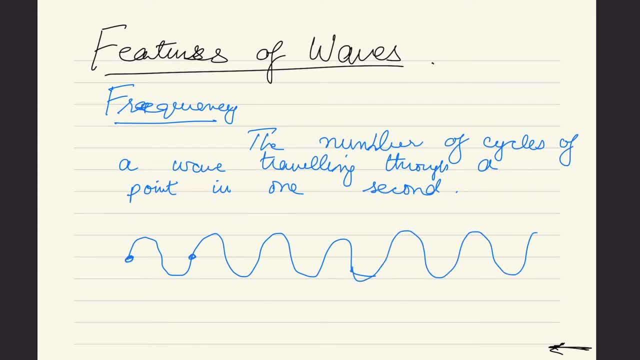 These are the cycles of the wave. One cycle starts from here, Ends here, Starts from here, ends here. Second cycle, third cycle, fourth cycle, Fifth cycle, sixth cycle. So let's suppose These six cycles are passing through A point. let's suppose The point is over here. point A: 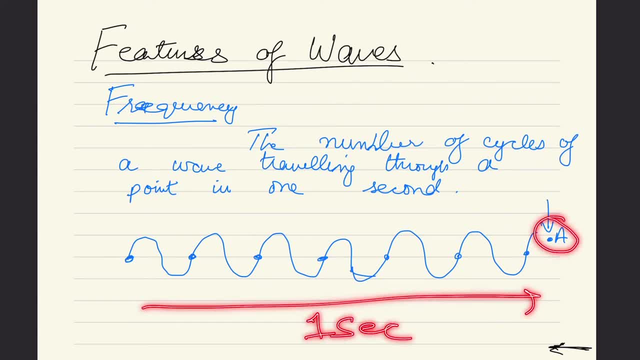 So let's suppose these six cycles Are passing through this point A In one second. The frequency of this wave Is Six hertz. Why six hertz? Because there are six cycles Passing Through A In one Second, So that's why the frequency Is six hertz. Hertz is the unit of frequency. 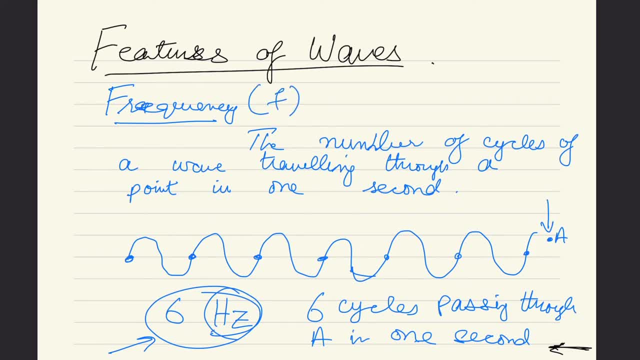 Let me just write it down over here With small f, And the unit Is hertz And we represent the unit with The symbol HZ. So that's how you'll explain The frequency. Now, the next thing that we have to discuss Is the time period. Is the time period? 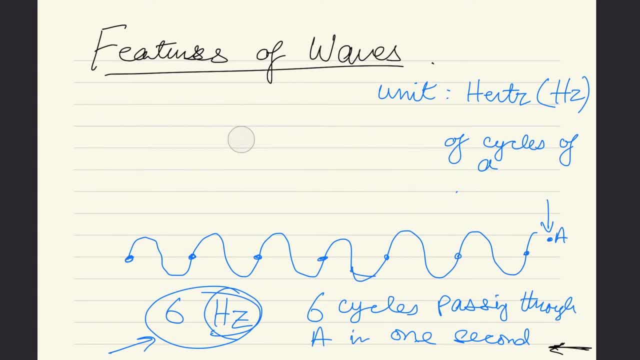 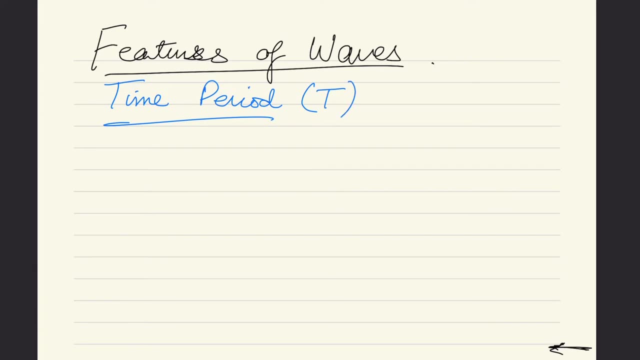 So let me just Raise it, Raise it, Raise it To The Time period. So the time period is Basically the opposite of the frequency. We represent the time period with T And, by definition, Time period is The time It takes For A wave To Complete one cycle. for example, we have a wave: 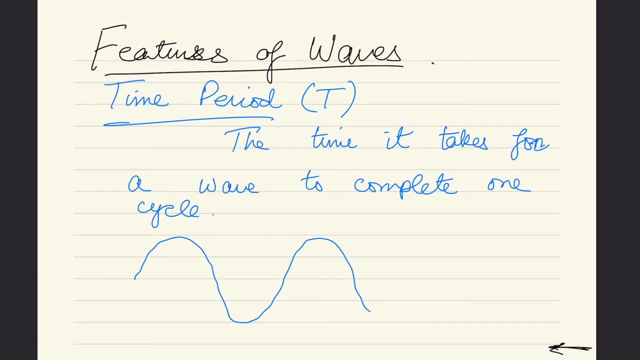 this is the wave. this wave starts from this point. it covers quarter cycle, half cycle, three, fourth of cycle and complete cycle. One cycle has been completed at this point. The time it has taken to complete this cycle, this first cycle, is the time period, For example. 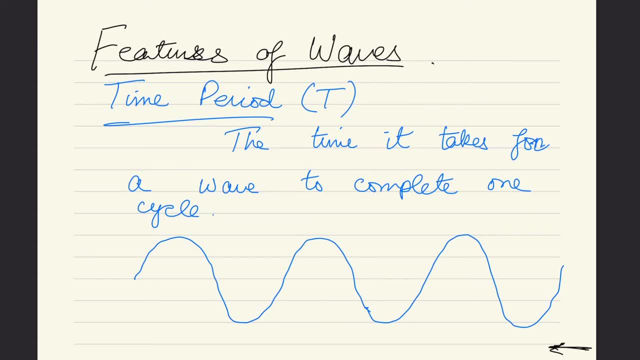 this wave took six seconds in order to complete these three cycles. so for one cycle it will be two seconds, or in simple words you can just say: the time it takes for a wave to complete one cycle is the time period of the wave. So the time from here to here. 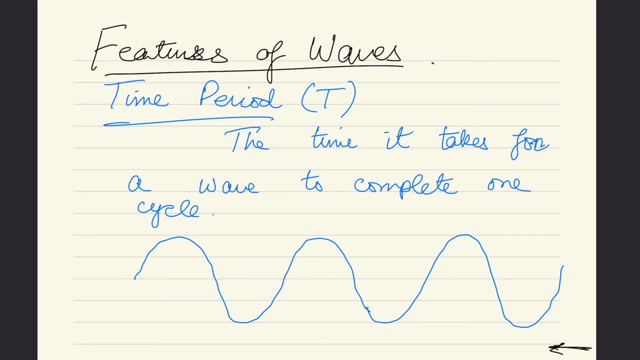 is the time period. we represent time with capital T, and let's discuss the relationship between the time period and the frequency. as I told you, that time period is opposite of the frequency, so let's discuss its relation. so frequency is equal to one over time period and symbolically we can write: F equals to: 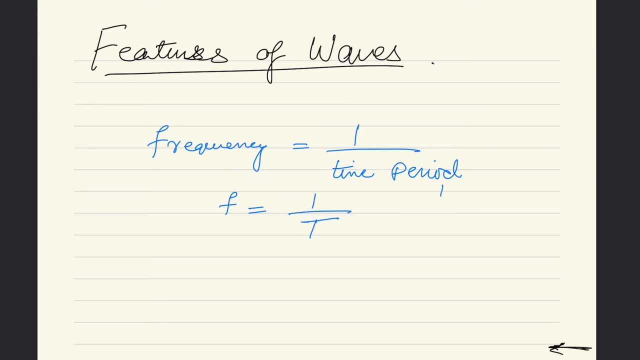 one over T and, by the way, the unit of the time period is seconds. We measure the time period in seconds. so if the time period is given in milliseconds or microseconds, or hours or minutes, we have to convert that into seconds. so that's the formula that relates the frequency and the time period. 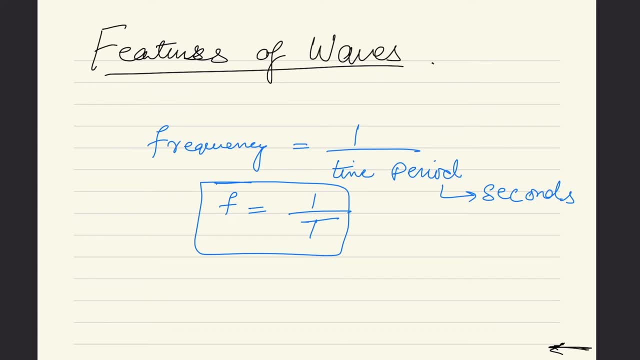 F equals to one over T, So this is the relationship between frequency and time period. Now, after that, we have to discuss about the wave speed. wave speed is simply the speed of the wave with which it travels, So wave speed is related with frequency and the wavelength. 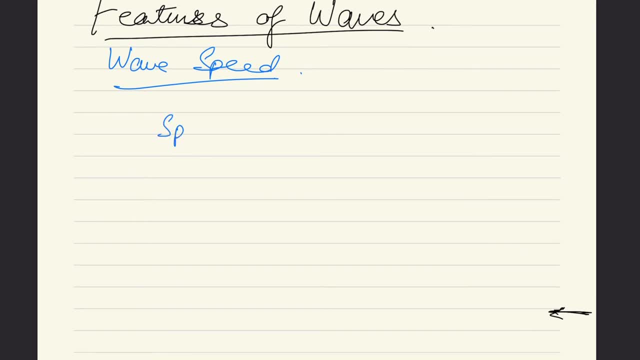 so we can write it as speed of a wave is equal to frequency multiplied by the wavelength, so V is equal to F lambda. So lambda is basically the symbol to represent the wavelength, and the unit of wavelength is meters, and V represents the speed, So V is equal to F lambda. 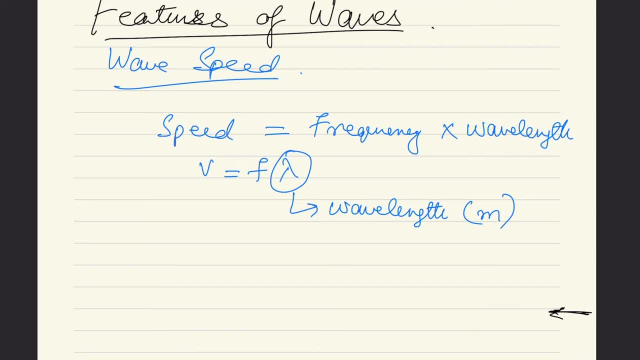 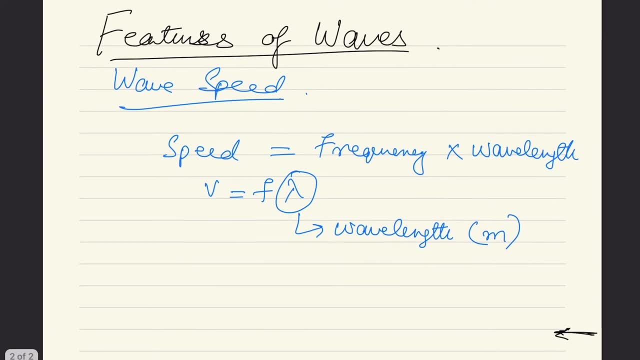 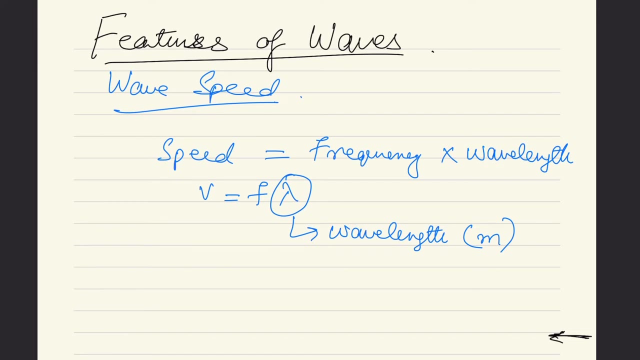 so this is the relationship of the wave speed with frequency and wavelength. So these are some of the features of the waves that we needed to discuss, and now we have to discuss about the transverse waves and the longitudinal waves. there are two types of waves: The transverse waves and the longitudinal waves. 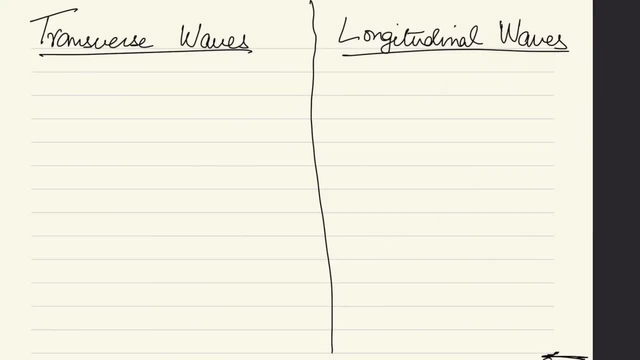 let's jump into that, Alright. so now we have to discuss the two types of waves: the transverse waves and the longitudinal waves. So lets write down the definitions first, and then I'll explain you What are the transverse waves and what are the longitudinal waves. So Transverse waves are the waves. 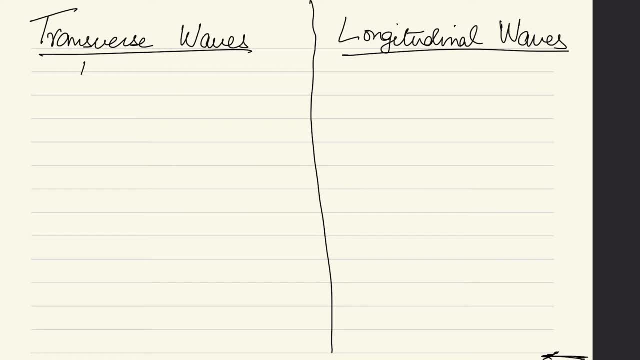 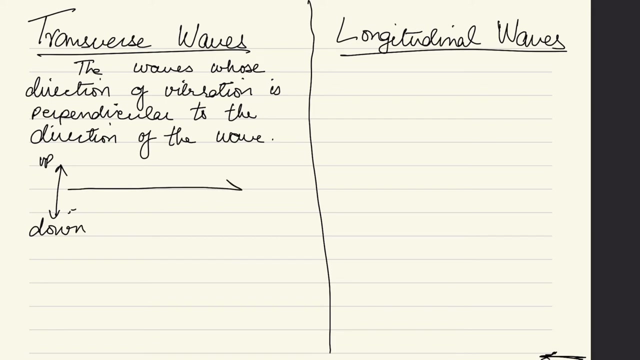 Whose direction of vibration is perpendicular to the direction of the wave. I repeat, the waves whose direction of vibration is perpendicular to the direction of the wave. For example, our wave is vibrating up and down, but the direction of the wave is to the right. 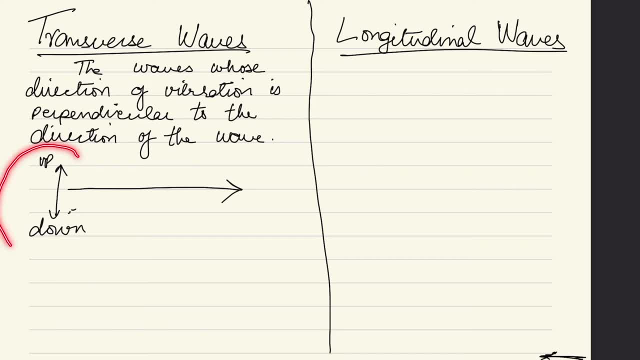 So you see, the wave is vibrating in the vertical direction and the direction of the wave is to the right. The vibration is in vertical direction, but the direction of the wave is in horizontal direction. So the wave itself is moving in the horizontal direction, but the vibration is up and down. 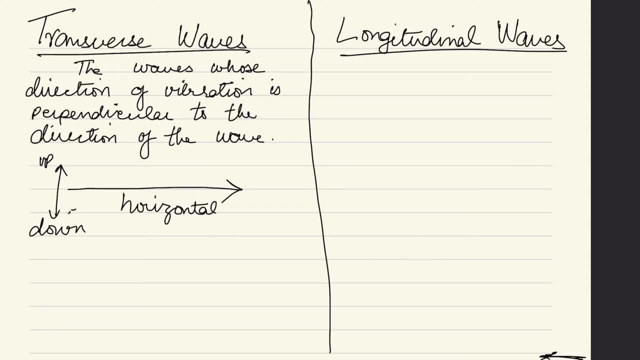 So such waves are the transverse waves where the vibration is perpendicular to the direction of the wave. Now, for example, all types of light waves are the transverse waves. Second, the water waves are also the transverse waves, And the waves in a string are also the transverse waves. 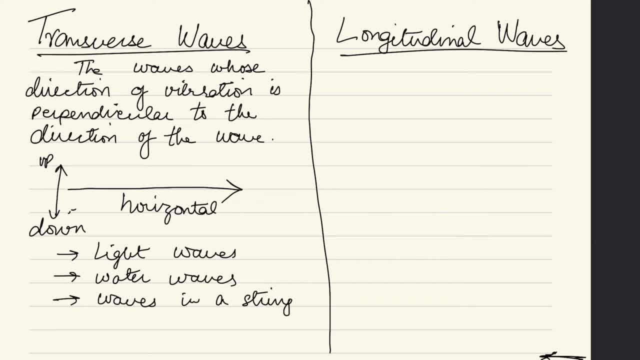 Moreover, we have the seismic waves. Seismic waves are the waves that are produced by the earthquake. So there are two types of seismic waves: S waves and P waves. Among those two types of seismic waves, the S waves belong to the transverse waves. 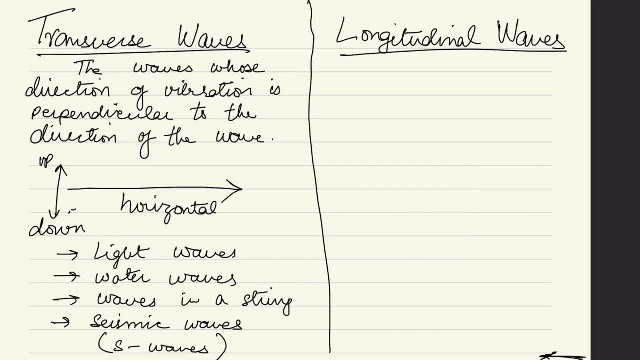 and the P waves. they belong to the longitudinal waves. I'll explain you. So: these are the transverse waves. So the most important thing that you have to remember in the transverse waves is this phenomenon: The direction of the vibration and the direction of the wave. 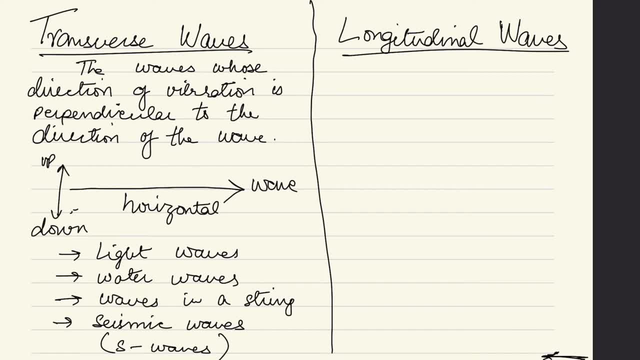 So the wave is moving in the horizontal direction and the vibration is up and down, So they are perpendicular to each other, which means it's a transverse wave. Now let's discuss about the longitudinal wave. So, by definition, the waves whose direction? 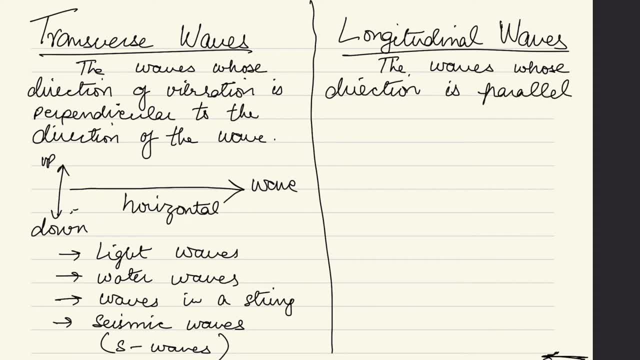 is parallel to the direction of vibration, So these types of waves are the longitudinal waves. For example, the wave is vibrating in the horizontal direction, So this is the direction of vibration, And the wave is also moving in the horizontal direction, So this is the movement of wave. 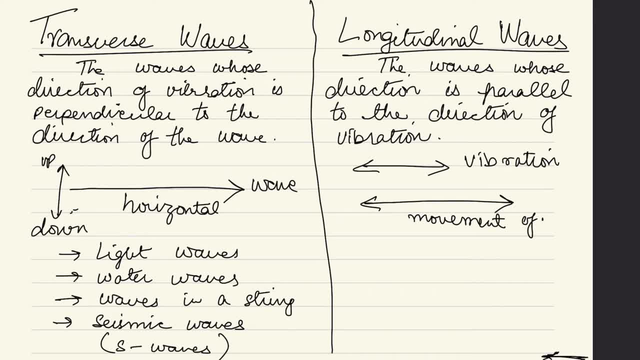 So you see, this movement is in the horizontal direction and that movement is also in the horizontal direction, So these two movements are parallel to each other. So such phenomena happens in the transverse waves. Such phenomena happens in the longitudinal waves. Now, the type of longitudinal waves are the sound waves. 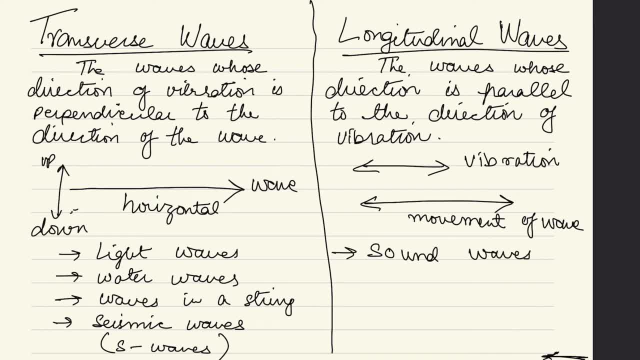 All type of sound waves are the longitudinal waves And the seismic waves. So from the seismic waves the p-type of waves are the longitudinal waves Right. So these are the differences between the transverse waves and the longitudinal waves Right. 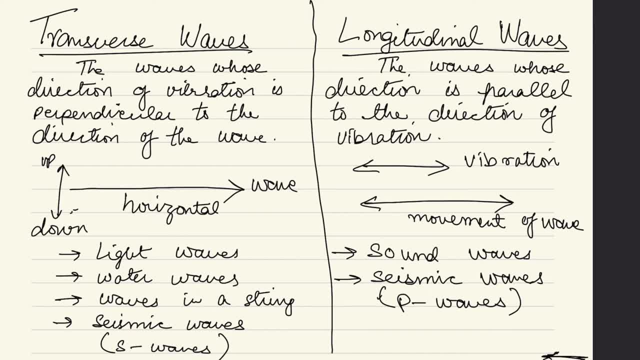 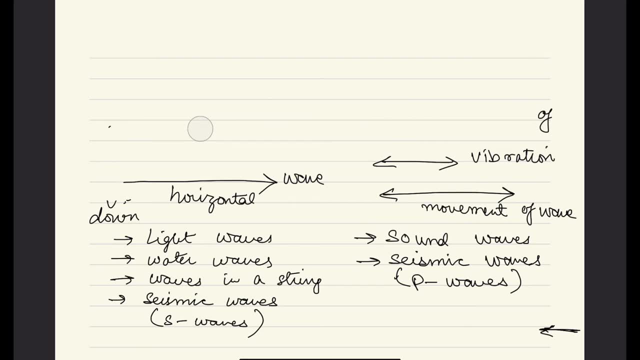 p-waves means like the primary wave, and s-wave means the secondary waves. All right, So this is it for the types of waves, All right. So after this we'll discuss some of the properties of the waves. So, in the properties of the waves, 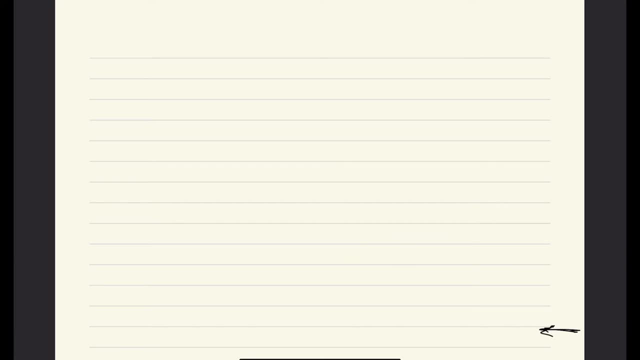 we have to discuss the behaviors of the waves. So properties of waves: Number one: waves can show reflection. Number two: waves can show refraction. Number three: waves can show diffraction as well. So these are the three main properties of the waves. 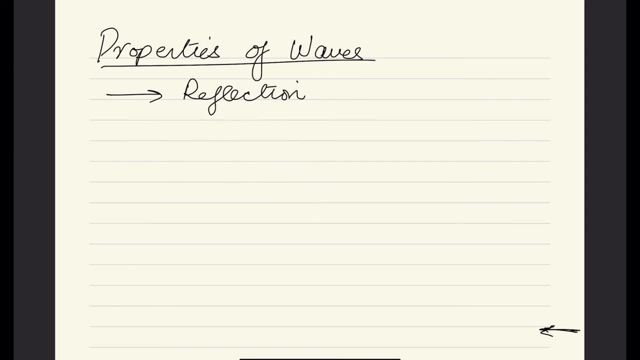 So let's see what is reflection. Reflection means, for example, this is a plane surface. A wave hits this wave hits this surface and bounces back. So this is the reflection. Okay, For example, let's discuss the water waves. 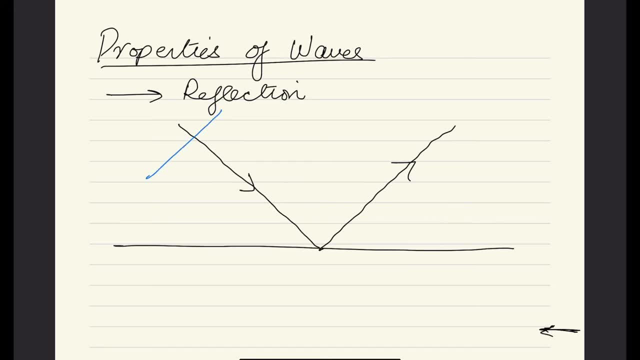 So I'm going to draw the wave fronts for the water waves. So these are the wave fronts of the water waves. So they are hitting this water surface and hitting this surface- This is the plane surface- and bouncing back. So 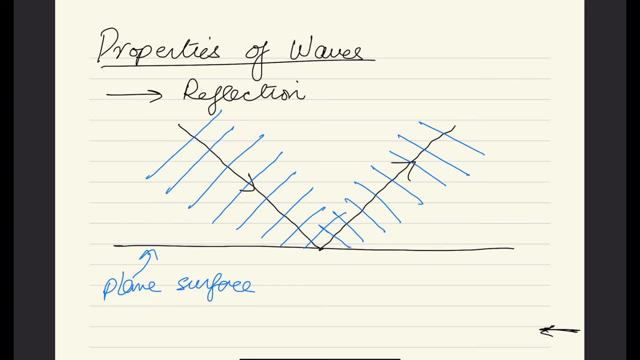 this plane surface has just changed the direction of the water wave, So this is the reflection. Now you can observe one thing: The distance between these wave fronts has not changed. The distance between these wave fronts is constant. So this is what happens in the reflection. 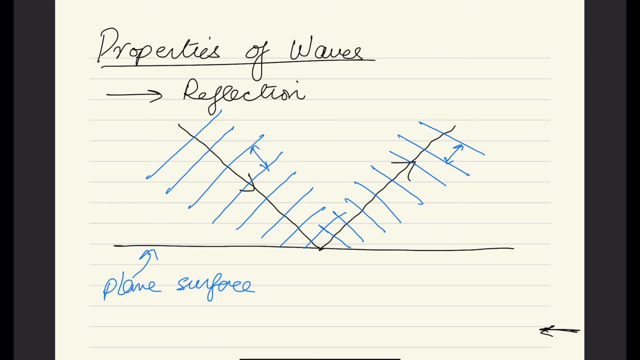 Because if the distance between these wave fronts change, it means its speed has changed. The speed of the wave has changed, But over here, since it's unchanged, which means the speed of the wave will not change under reflection. Now the next phenomena that we have to discuss is: 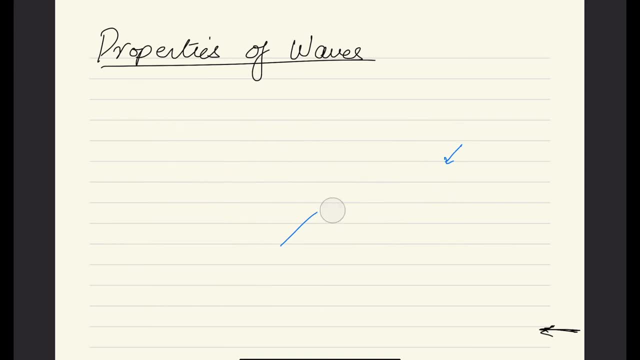 refraction. So in refraction what happens is a wave. let me use black color. a wave enters from one medium to another. This is basically the refraction. So when a wave changes its medium. let's suppose a wave enters from air- 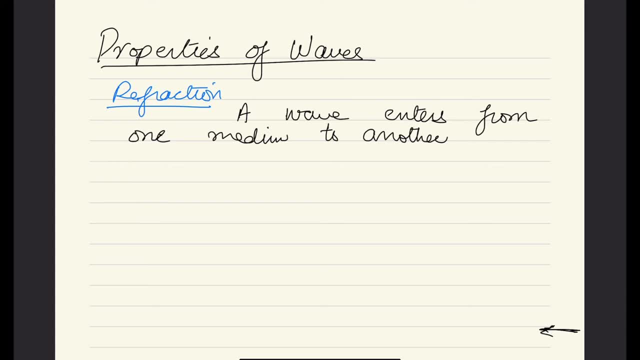 a light wave enters from air into the glass, air into the water, air into the diamond, you know. So its behavior will change. By behavior I mean its speed will change, Its frequency will change. Frequency will change, as I said. 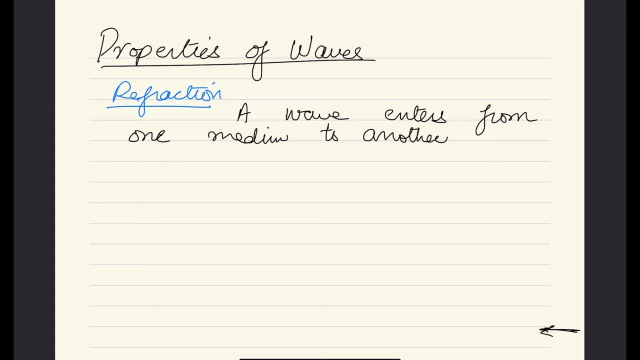 the wavelength will change. So when a wave enters from one medium to another, that's called refraction. So we have a medium over here. So let's suppose this is a glass block And over here we have air. 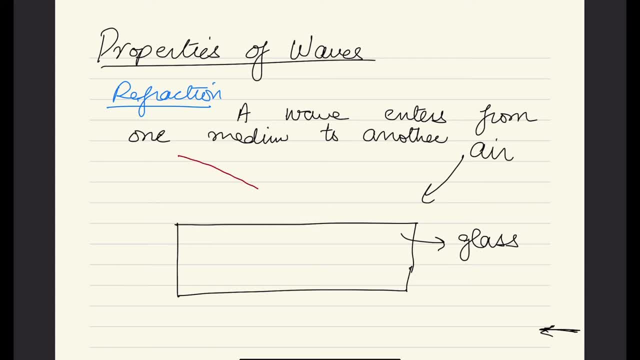 A light ray enters from air into the glass. So this is the surface, this is the boundary of the glass. Now, instead of moving straight, it will not stay straight. It will bend a little bit. It will show some bend like that. 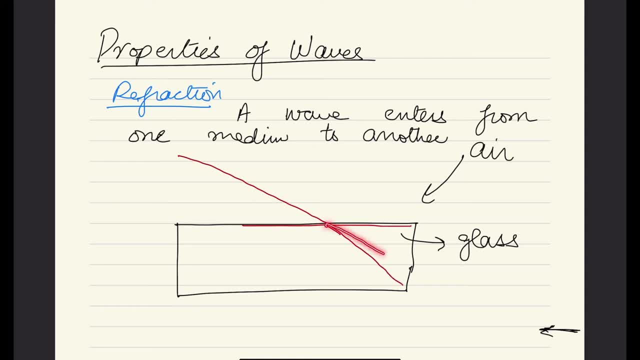 So it was supposed to move straight but it has shown some bend. So this is basically refraction. So when a wave enters from, when a light wave or any other wave enters from one medium to another, its direction changes. 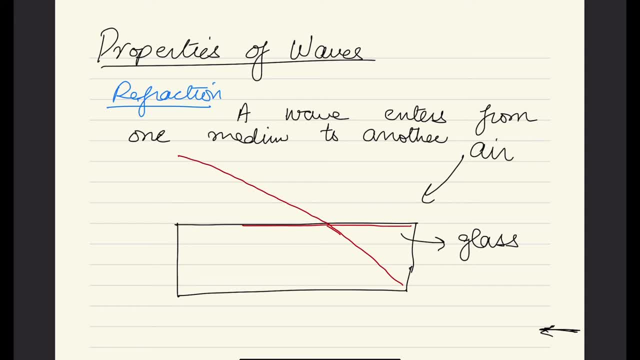 Its speed changes depending on the type of material in which it entering it is entering. We'll discuss it later on in the topic of light, But for now, just to get an idea, refraction is basically when, a when a wave enters from one medium to another. 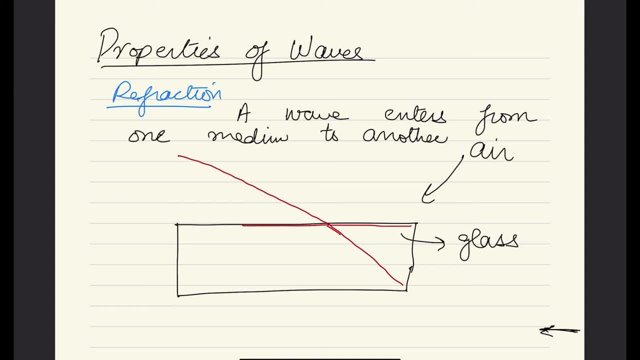 That's the refraction. Now, the next thing that we have to discuss is diffraction, Diffraction. So diffraction is basically: it is the spread of a wave when it escapes from a narrow opening. That's the diffraction. 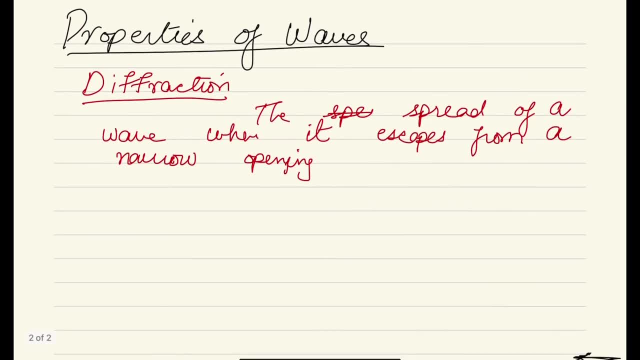 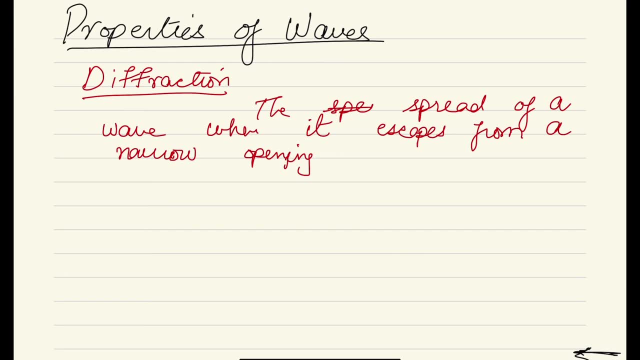 Alright. So the spread of a wave when it escapes from a narrow opening is the diffraction. For example, there's a light wave and this is a small narrow opening Right over here. that's a small narrow opening, A light ray. 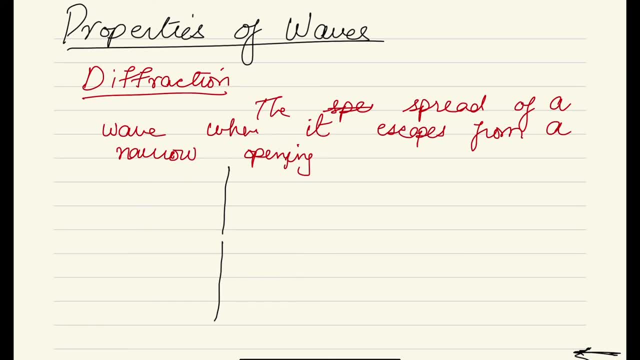 is coming over here, For example, there's a light ray that's coming over here, Right over here, So there's a light ray coming over here. So, after passing through this narrow opening, this light ray will spread. It will spread. 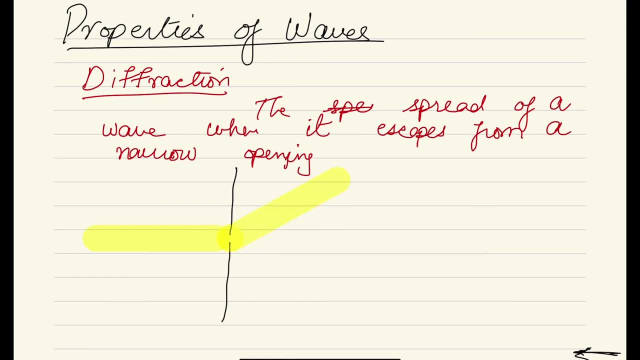 like this. So the spread of the wave is called the diffraction. Obviously this is a bit inaccurate figure. Let me just correct it. So it will spread from this narrow hole like that in all the directions. So this spread. 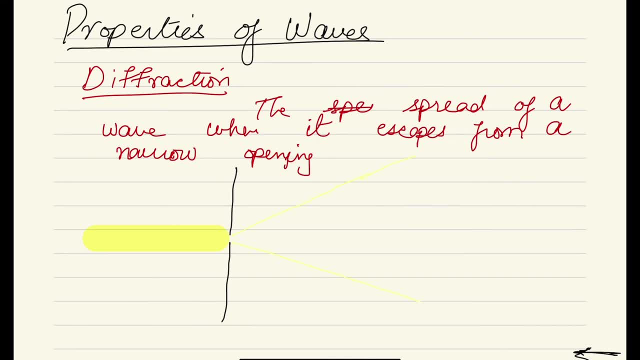 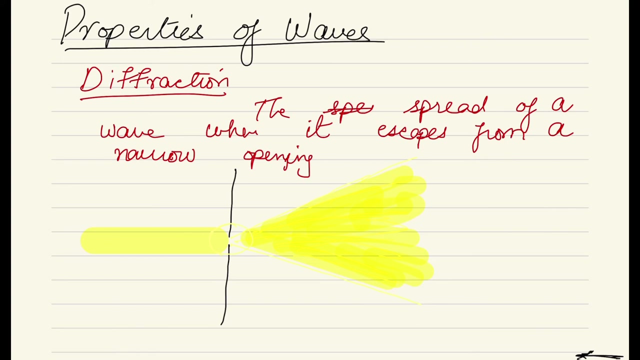 will spread from this narrow hole to this narrow hole. So this spread is represented by diffraction. There you go. So in this way, the waves diffract. Now we'll discuss how this narrow hole affects the diffraction of the. 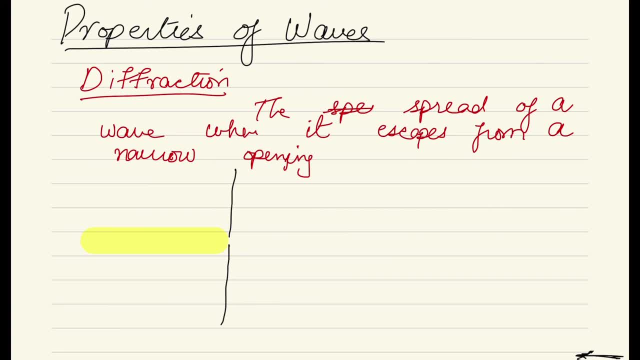 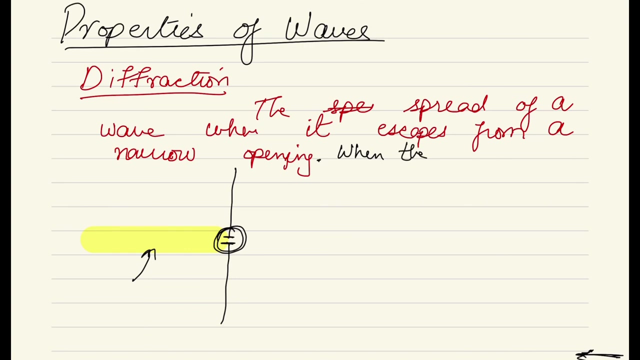 wave. So if this narrow hole, if this opening right over here, if the size of this opening is equal to the wavelength of this narrow hole, narrow opening is equal to the size of the wavelength, In that case the spread will be. 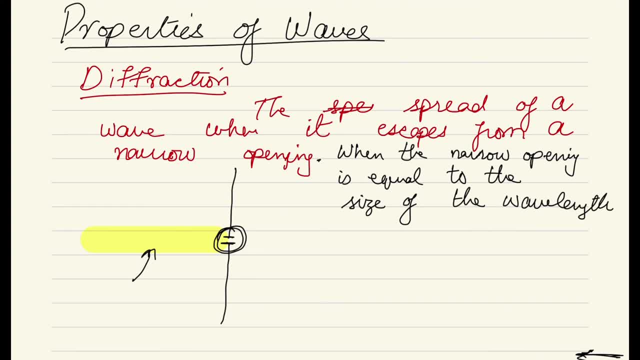 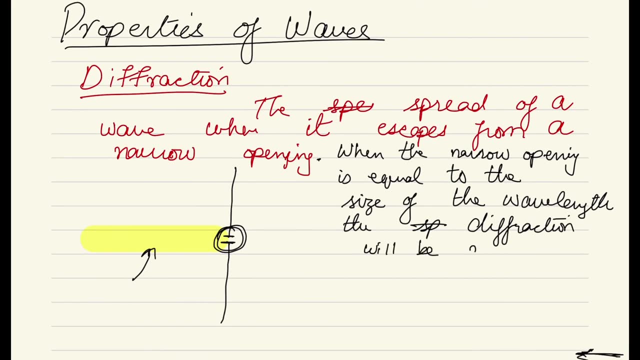 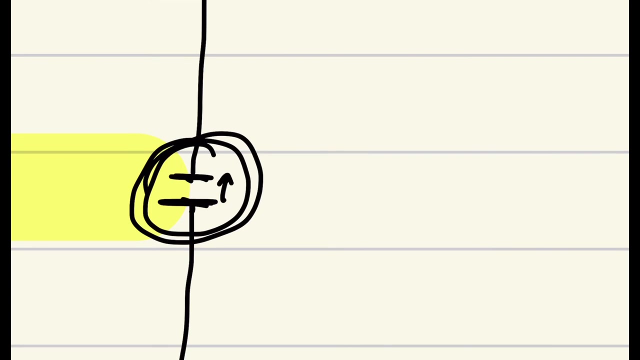 maximum, or we can say the diffraction will be maximum. For example, the length of this narrow opening is L. Okay, So if the length L is equal to the wavelength lambda, in that case the diffraction will be maximum. 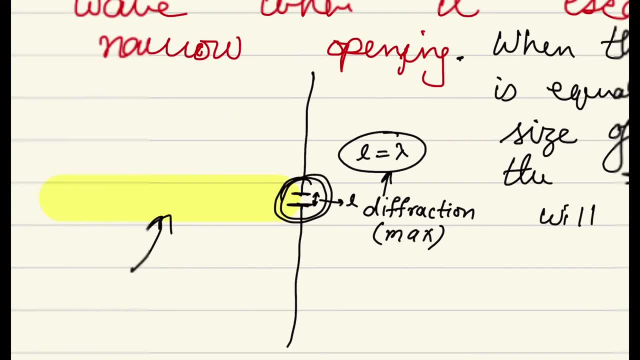 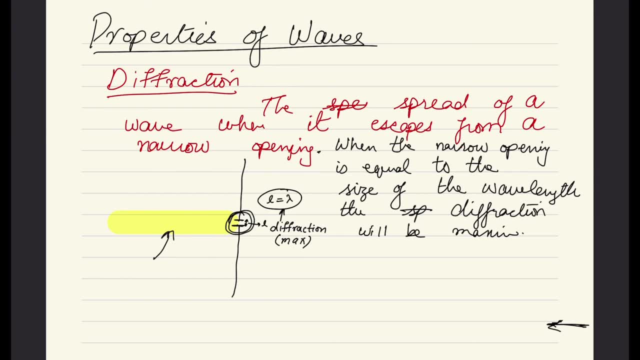 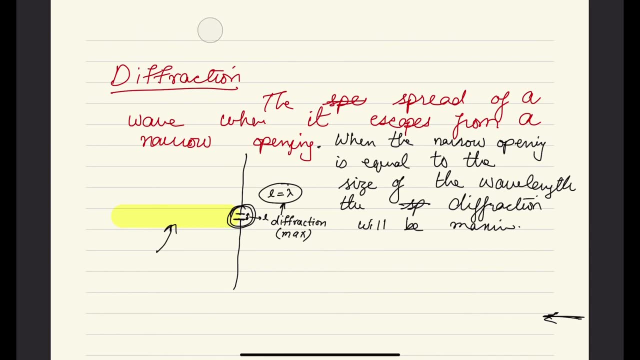 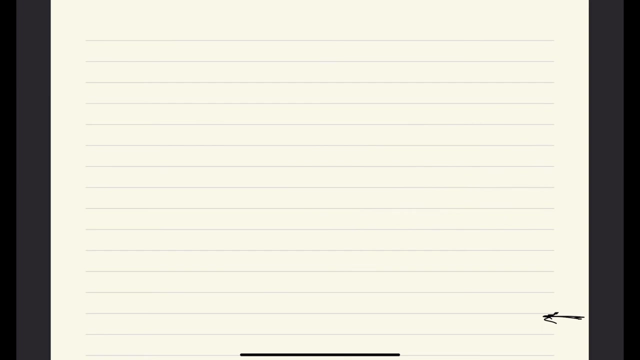 Alright, So that's how you can tell about the diffraction of a light, of any wave, basically Okay. so now we'll discuss some more properties of the wave by drawing a graph. So it's a tank with a. 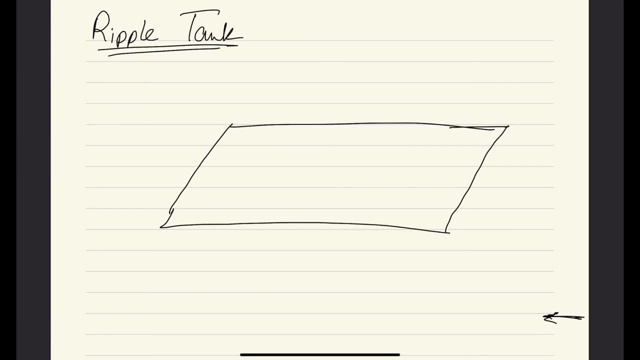 top, where there's a transparent sheet at the bottom And there's a light lamp at the top. There's light coming from here And there's a white sheet at the bottom. That's the white sheet at the bottom And we have the. 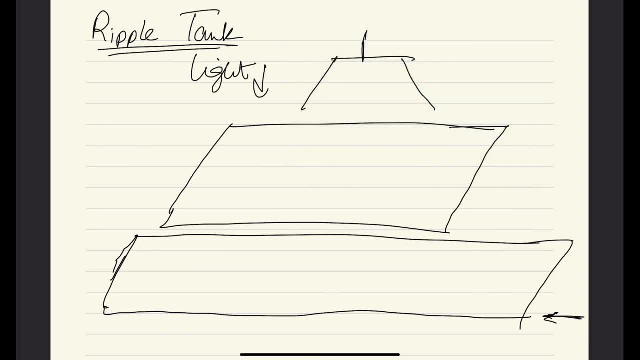 water waves over here. I'm just drawing the wave fronts of the water waves, So these are the wave fronts. Now, these wave fronts, let me just redraw the wave over here. Let's suppose this is the wave, So these. 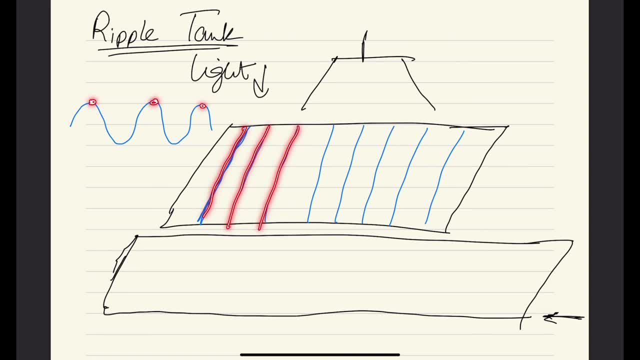 lines over here. they're representing the crests of the wave, And that region is the trough of the wave. Now, when the light turns on, it falls on these water waves, And wherever there are wave fronts, we will see some dark. 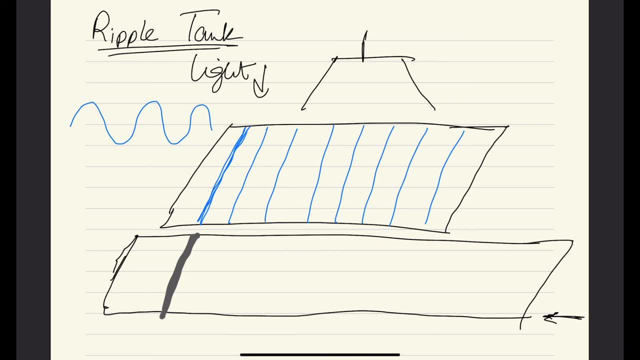 regions. See over here. So these dark regions are being shown on this paper sheet, on this white sheet. So these dark regions are representing the crests of the trough. Now, if you want to measure the wavelength for that purpose, 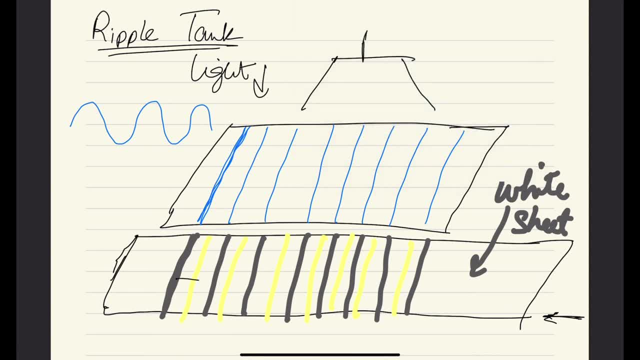 we just have to measure the distance between any two consecutive dark regions. So these are the wavelengths. So now let's do some alterations in this ripple tank Over here till this region, the length of the you can say the depth. 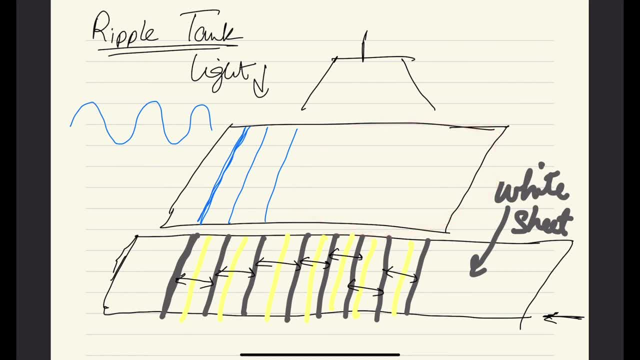 of the ripple tank is more and over here. remember, depth is more over here and depth is less over here. So now I'm gonna make some changes in the wave fronts and you'll observe those changes, So I'll. 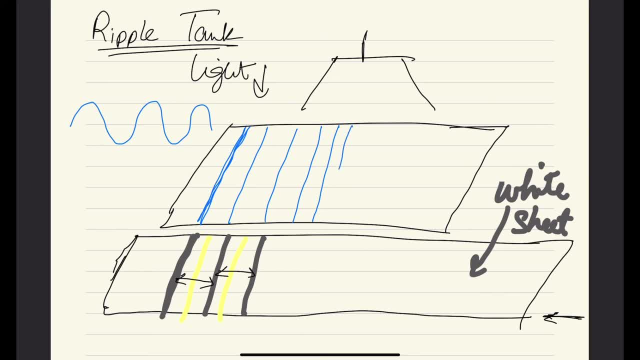 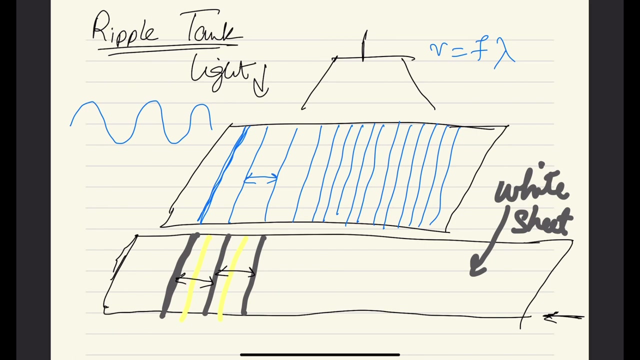 also remove these lines as well. All right, So I'll remove these lines like that. These are the wave fronts, All right. What does it say? We know that v is equal to f lambda, So you see over here. 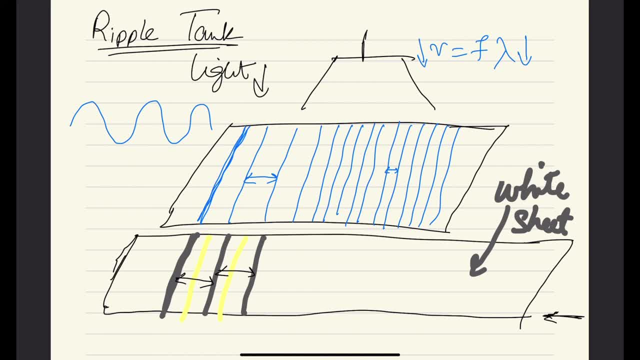 the speed of the wave will also decrease. Why? Because the wave fronts become close to each other and the wavelength decreases. As the wavelength decreases, so that the speed of the wave will also decrease in the distance between these dark lines. So 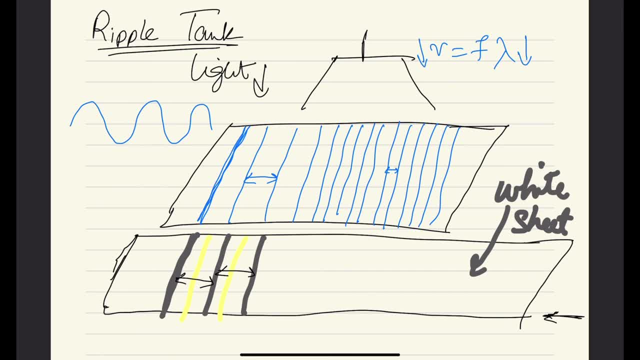 the distance between these dark lines has decreased, which means the speed of the wave has decreased, So the distance between these dark lines has decreased. So as a conclusion, we can say that I'll just write down my conclusion over here. Let me 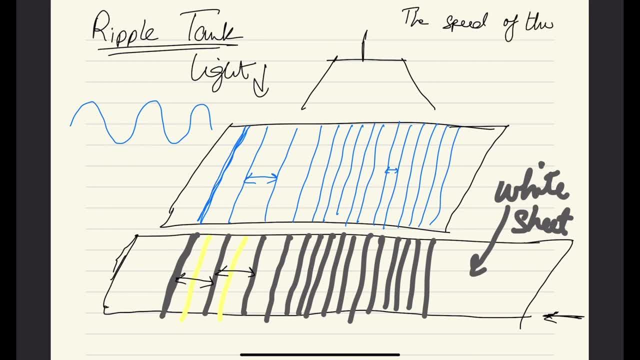 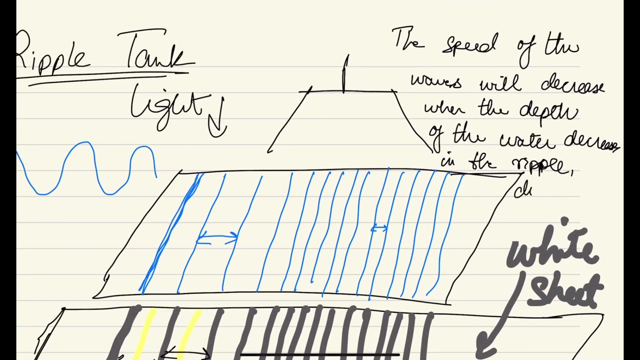 just find some space over here. The speed of the waves will decrease as the speed of the water decreases in the ripple tank. And why does it happen? It happens due to decrease in the ripple tank, And why does it decrease in the wavelength? 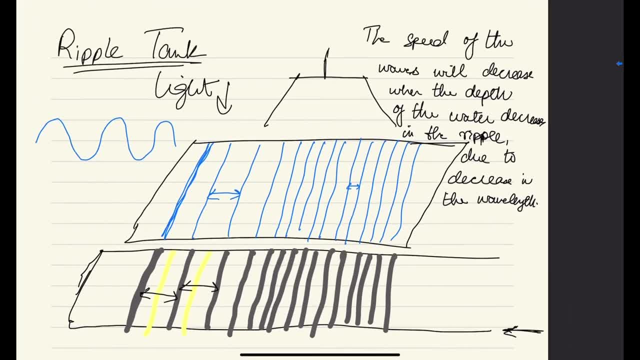 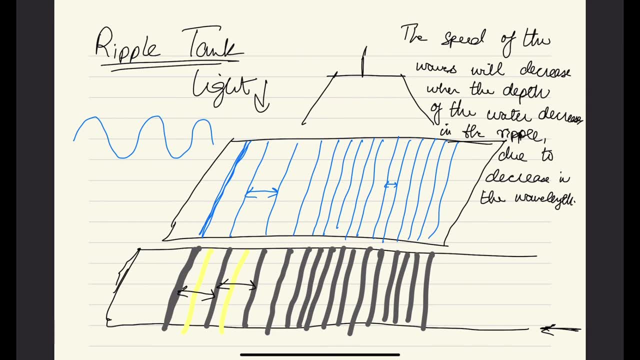 So that's the whole story of the ripple tank. I hope you got it. So this is it for the next video. Thank you for watching. See you in the next video, Thank you.